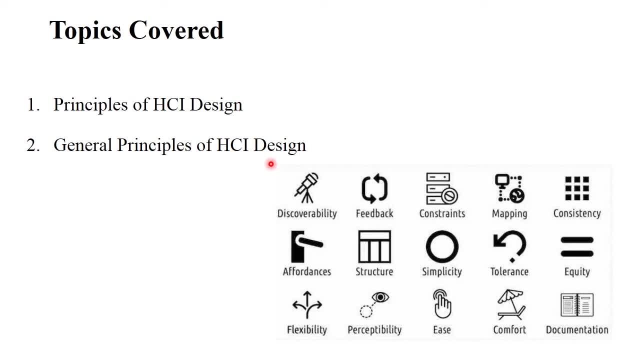 and general principles of human-computer interaction design. This image just shows the symbols of each and every principles like discoverability, feedback, constraints, mapping, consistency, affordance, structure, simplicity, tolerance, equity, then flexibility, perceptibility, ease, comfort and documentation. 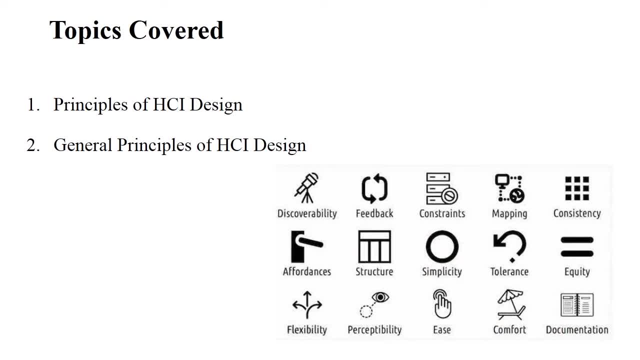 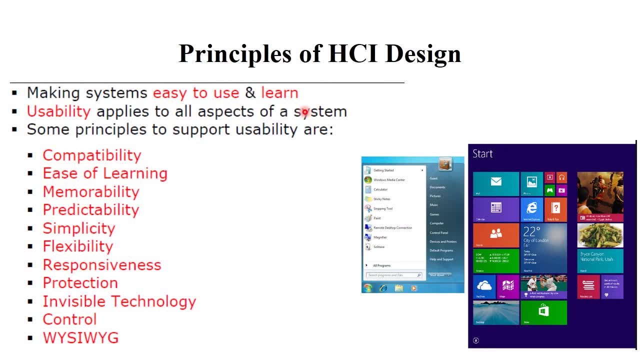 So let's see, one by one, how each and every principles are work. Okay, next, Principles of human-computer interaction: design. These principles which makes the system more easy. These principles which makes the system more easy. These principles which makes the system more user-friendly, easy to use and easy to learn. 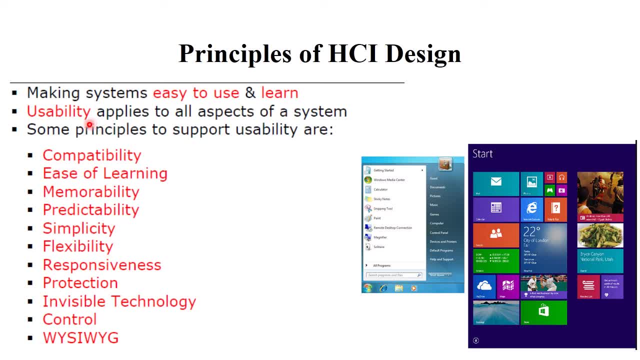 Okay, I already told you in my previous video: usability. Usability is one of the most important principles of human-computer interaction. Usability applies to all aspects of a system. Usability applies to all aspects of a system Because each and every generation, each and every person. 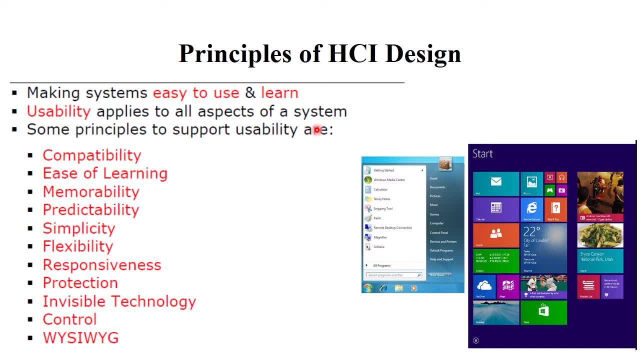 whether it is technical people or non-technical people, whether it is technical people or non-technical people, each and every one use the computers. That's the usability Clear. There are some principles that supports usability, which includes compatibility, ease of learning, memorability, predictability, simplicity, flexibility. 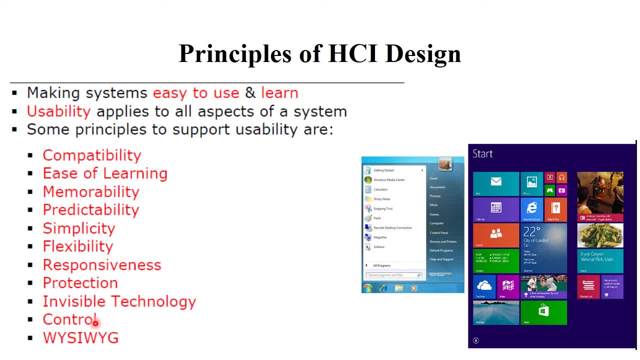 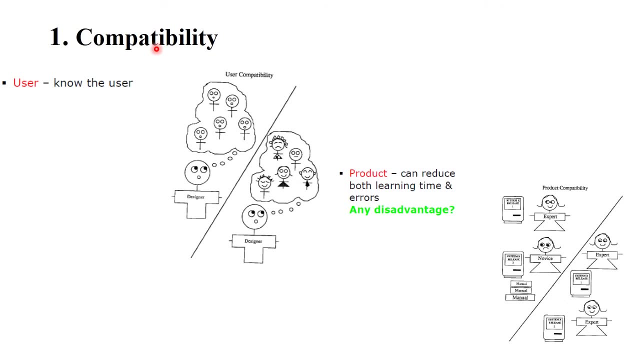 responsiveness, protection, invisible technology, control and w y s i w y j. okay, so let's see one by one how these principles are work, okay, next, so first principle of human computer interaction is compatibility. okay, see here, when you have to develop a particular product, so you must know. 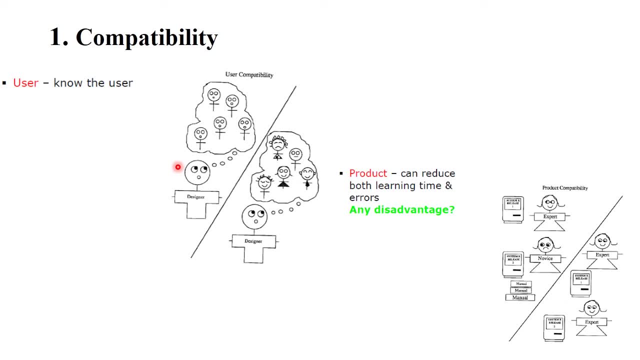 your customer or your user, okay. so first principle is user, that is, know the user. okay, it's your responsibility to know the education purpose, intention, then age group, their field, this, each and every information about your customer, about your user. you must know the requirements, What exactly requirements and what is the need of the user. 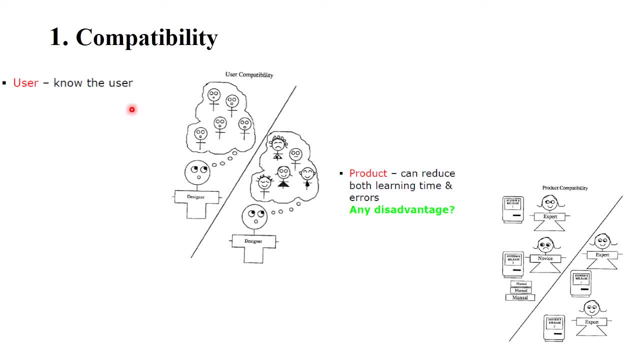 Okay, So this is the first principle of human computer interaction, that is, compatibility regarding to the user. Clear, The goal of the designer, or goal of the developer, is to satisfy the user, their user. Okay, All the customers are happy, Then your product is become very quality, full. 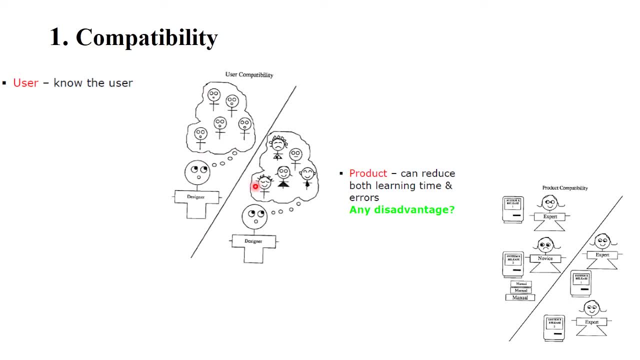 Clear. Okay. Now see in this diagram, all the persons in this diagram are very happy Regarding to that particular product, Okay, But here there are different types of people, different types of emotions are there, Okay, So you must focus on your customers are become happy through your product. 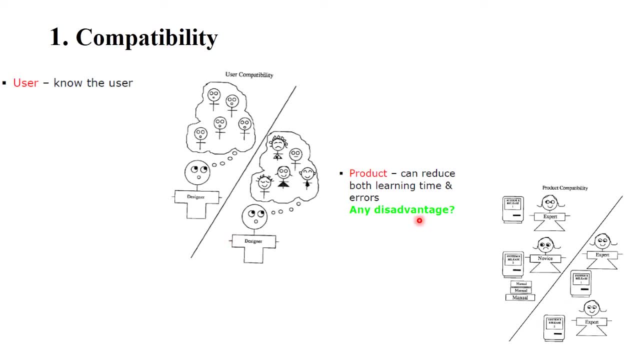 Clear. So this is a compatibility mode And second one is product. Product means it can reduce both learning time and errors. Okay, We all are familiar with space complexity and time complexity features Right. So when you have to develop a particular product, 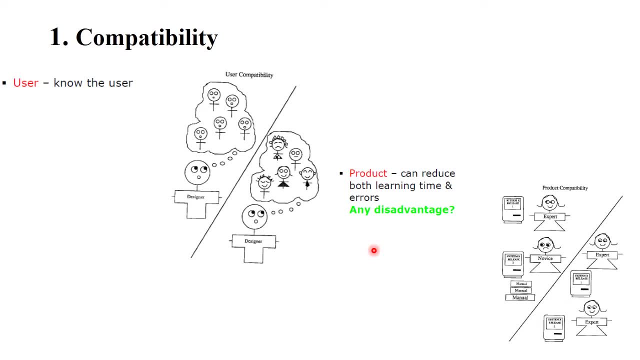 Whether which has less space complexity and less time complexity- Okay, In minimum time the product can be run Okay- And which required less space- Clear. So this is called as product And this is called as compatibility Means you have to compatible with your user and also with your product. 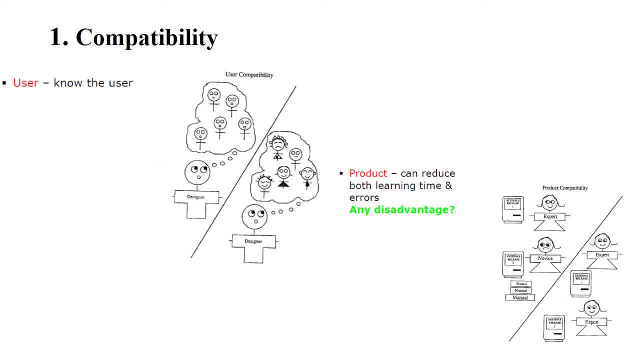 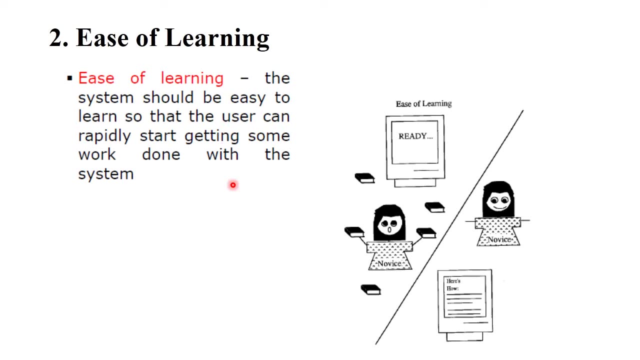 Clear. This is the first principle. Next, Next, Next principle is ease of learning. Okay, The system should be easy to learn So that users can rapidly start getting some work done with the system Clear, For example, when you have to use particular app. 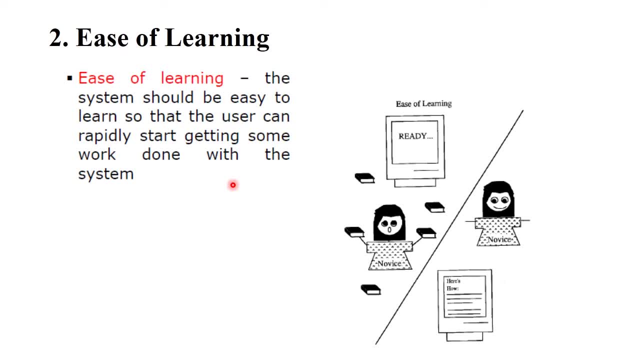 For example, WhatsApp, Okay, The each and every features are directly denoted: The chat functionalities, audio video calling, the contact list, etc. So it easy to learn for each and every person, Whether it is technical or non-technical or any other age group. 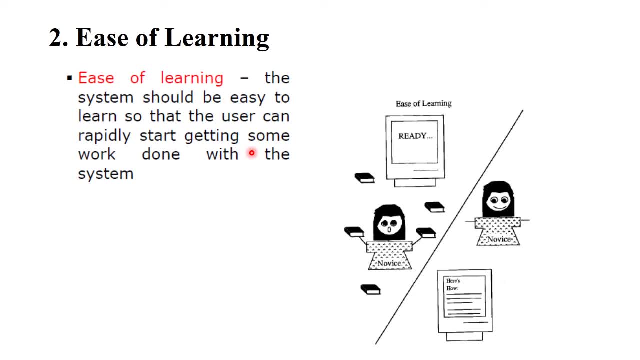 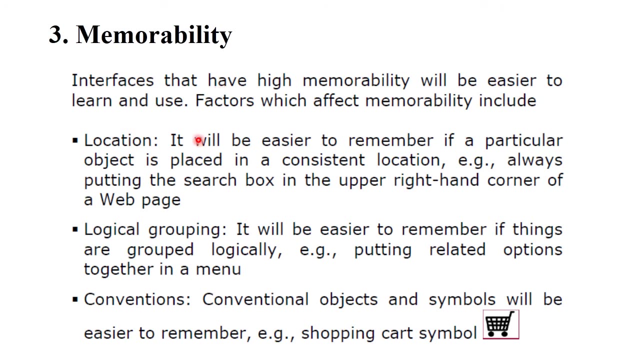 Okay, So this is the ease of learning. So this is the second principle of human-computer interaction. You must follow this principle. Clear, Okay. Next, The third is memorability. Okay, This is the third principle of human-computer interaction. 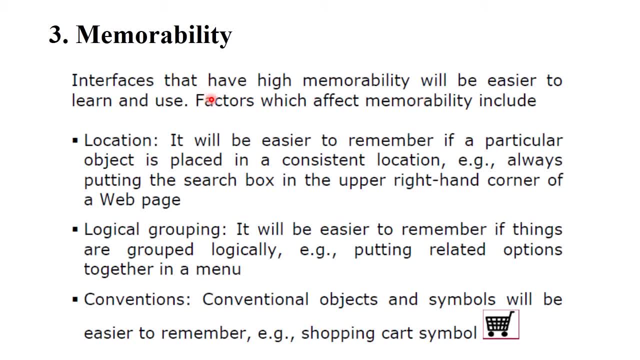 Interface that have high memorability will be easier to learn and use. Factors which affect memorability includes There are three factors: Location, logical grouping and convention. Okay, So first, what is meant by location? Location: it will be easier to remember if particular object is placed in consistent location. 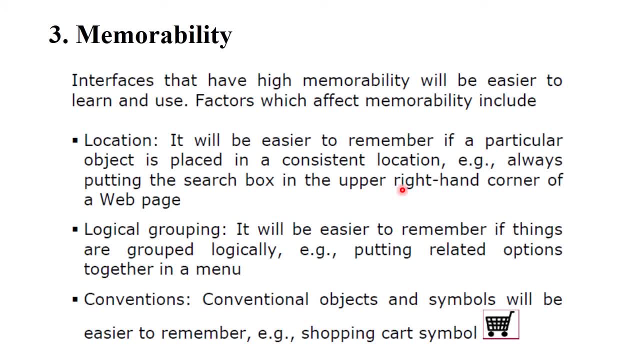 For example, always putting the search box in the upper right hand corner of web page. Okay, For example, when you use Microsoft Word. Okay, There is page layout option. Or in this page layout option, there are page border, page setup, page number. 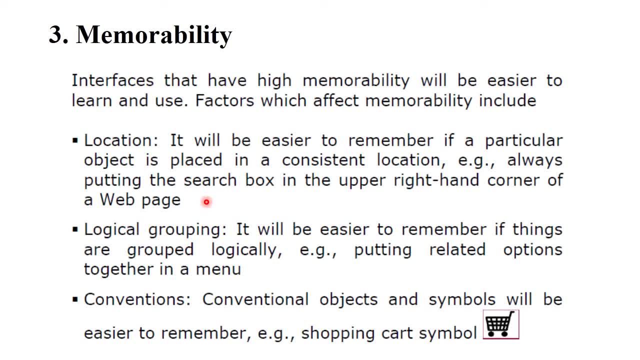 These kind of functionalities are included. So this is called as proper location of that particular function. Clear, So it is easy to find or easy to use. The next one is logical grouping. It will be easier to remember if things are grouped logically. 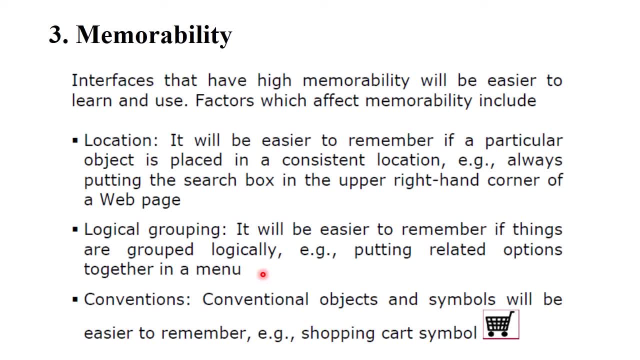 For example, putting related options together in menu Clear Next conventions. Conventional objects and symbols will be easier to remember. For example, shopping cart symbol. Okay, Sometimes symbols denote one of the most important part. Okay, In Microsoft Word there will be copy paste. 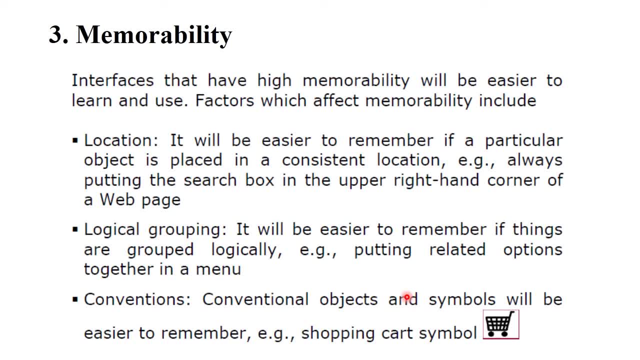 Okay, Then new files are open. These kind of symbols are available in menus Right. So through these symbols you can also work, or you can also use these symbols Clear. So this is called as memorability. Memorability includes location, logical grouping and conventions. 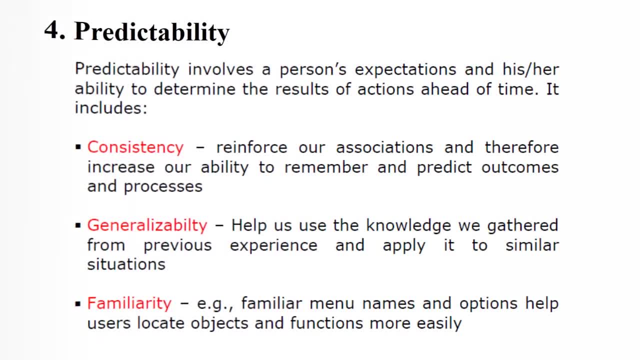 Clear Next. Next is predictability. Okay, This is the next principle of human computer interaction. So predictability involves a person's expectations And his or her ability to determine the result of actions ahead of time. Okay, Predictability includes consistency, generalizability and familiarity. 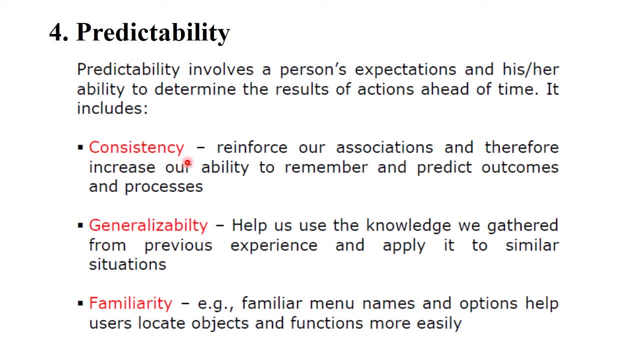 So what is meant by consistency? Consistency, reinforce our association and therefore increase our ability to remember and predict outcomes and process. Okay, This type of functionalities, suppose, you have to add in your product, then this type of outcomes will be generated. 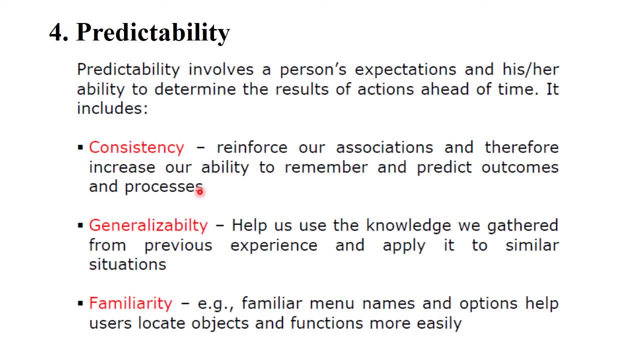 This is called as predictability- Okay, This is called as consistency- Clear, Next, generalizability. It helps us to knowledge we gathered from previous experience and apply it to the similar situation. Okay, For example, there are different types of products are generated. 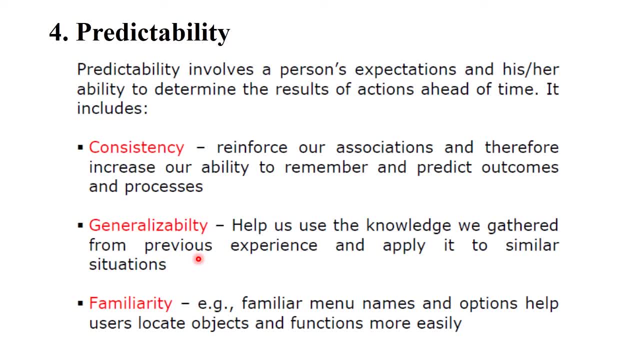 Okay, There are different versions of that particular products are generated, Clear. For example, in alpha version different functionalities are added, But in beta version these functionalities and also some other functionalities also included. This is called as generalizability. Okay. 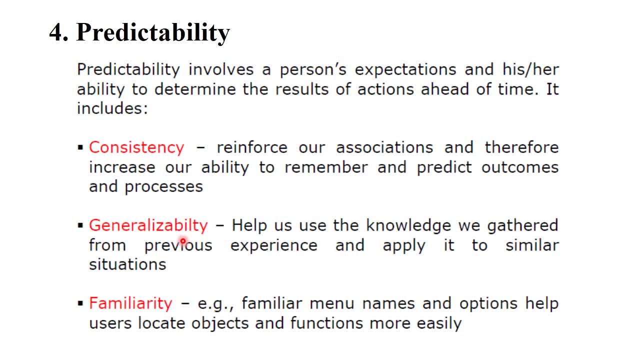 The another word of generalizability is inheritance. You all are familiar with inheritance- Clear. Okay. The next is familiarity. For example, familiar menu names and options help user locate objects and functions more easily. Okay, In Microsoft word, for example, the new cut, copy, edit, paste- this kind of words are used. 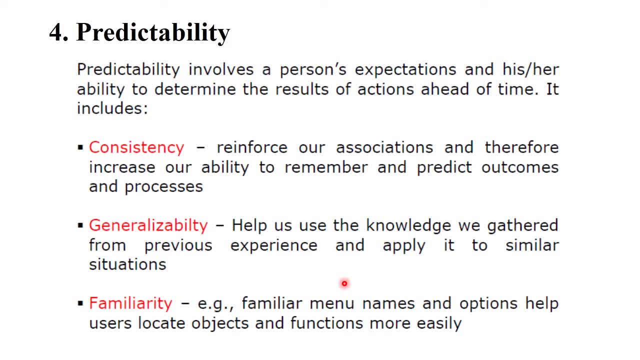 And this kind of words is more familiar to the user. Okay, So this is called as familiarity. Don't use much difficult word. Okay, Use the word very easy to understand for each and every people. Clear. So this is the principle of human computer interaction, of predictability. 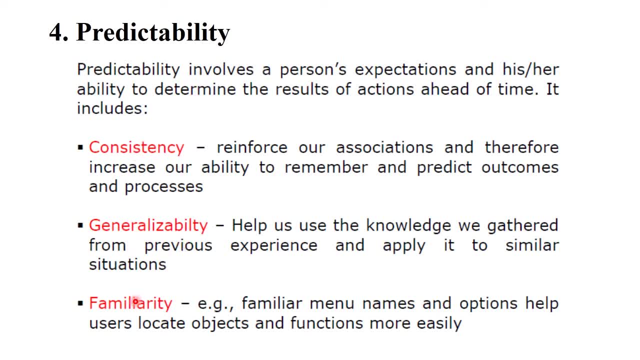 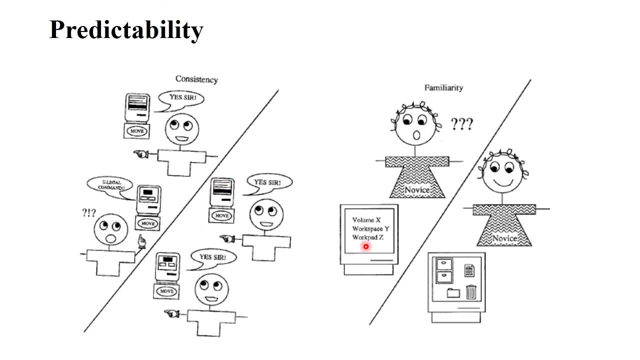 So predictability includes consistency, generalizability and familiarity. Clear Okay, Next Okay. This is just example of predictability. Here, users are in very consistent mode, Right, And your customers are also in familiar mode, Okay. 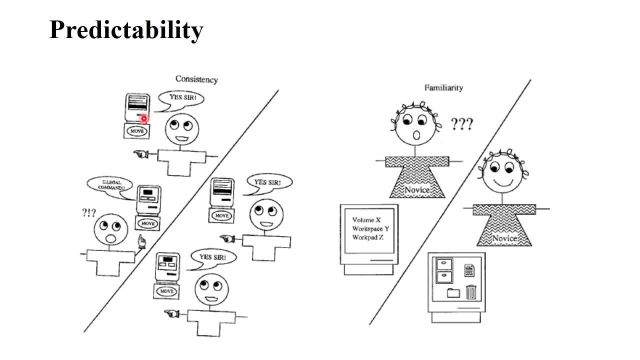 Consistency is related to the CPU or your system. Okay, Their space complexity, their time complexity- This is the consistency of the system. And now familiarity is related to the user. Clear, This is just difference between consistency and familiarity. Consistency is related to the system and familiarity is related to the user. 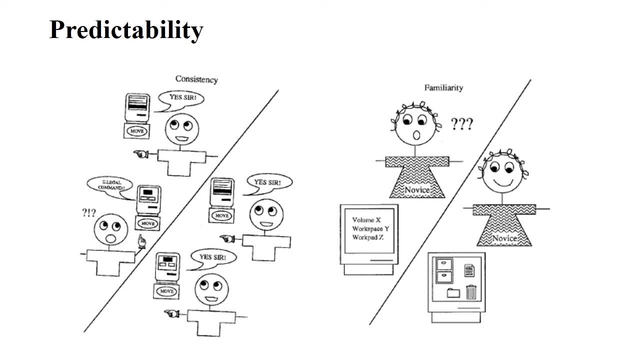 User is familiar. I wanted to come to this point, So now we'll come to convenience and constancy. Consistency here means theե�. Consistency is important here. Consistency is Anger And COM is there, which is like anger escaping inner binary, which is like tie pleasantness. 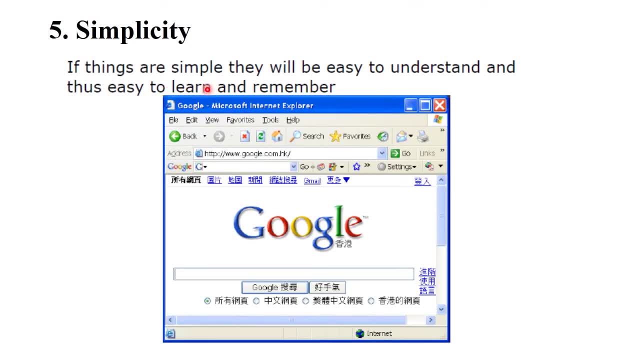 good Consistency. isamb dess. Consistency is one of trend mentality, So its something to consider carefully. So I think these three are the eight typical Society of Cons, muscles and Hell, envin And podia. What is the society of Cons- muscles? 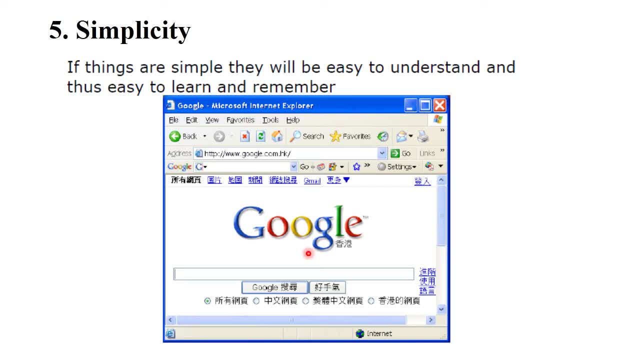 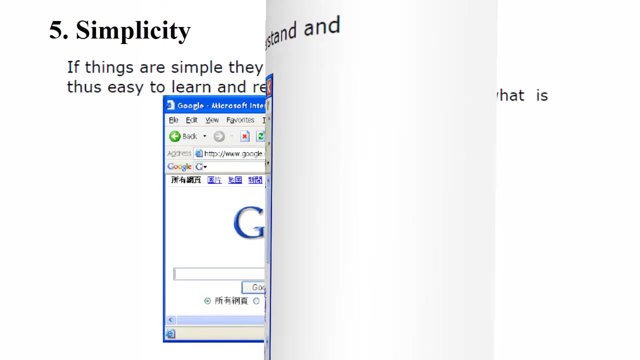 Andhall Are Humor, Agenda, Cognition, Consistency, Consistency, Confidentiality, particular surface, clear. so this is called as simplicity. when you will develop your product, your product is more simple. okay, then each and every persons are used this and enjoy your product. clear, okay. next, this is another. 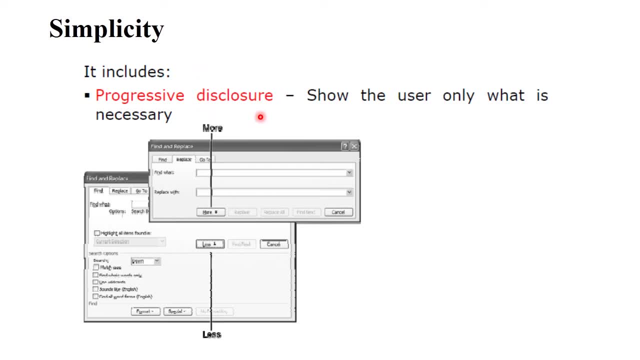 example of simplicity. it includes progressive disclosure. show the user only what is necessary. okay, see here in this dialog box there is more option. is here? okay, but when you click on more option, then this kind of dialog box is open. okay, so this is called as. progressive disclosure means show the. 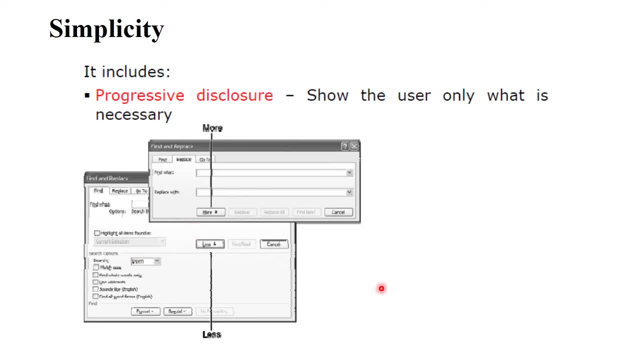 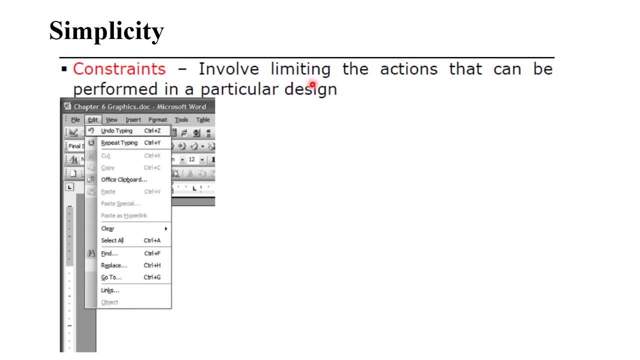 only that information user need. okay. next, this is another example of simplicity, that is, constraints. it involves limiting the action that can be performed in particular design. okay, for example, in Microsoft Word, there is edit option. in edit option, when you click on edit, you will see that there is a dialog box which is called as progressive disclosure. 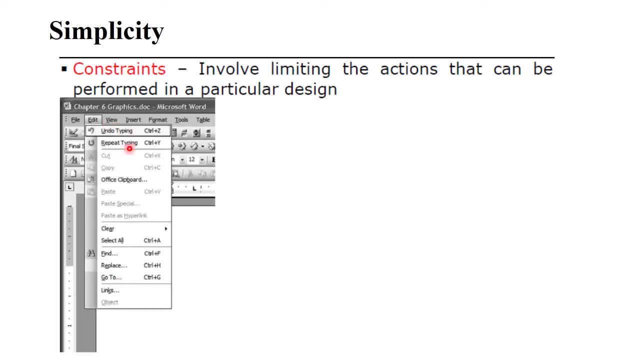 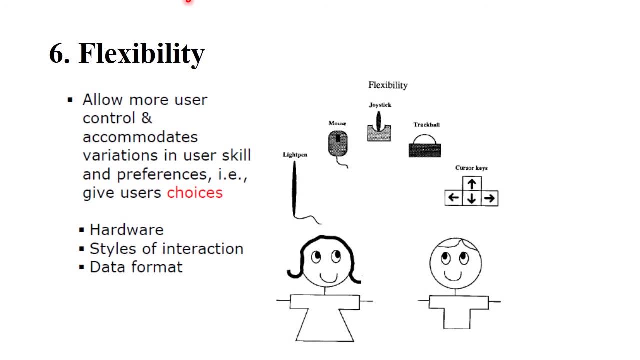 there are different types of menus are included: right the undo, typing, repeat, typing, clear, select, all, fine, replace, go to, etc. so this is called as constraints: okay, so it involves or it included in this edit option: clear, okay. principle of human computer interaction is flexibility. flexibilities allow more. 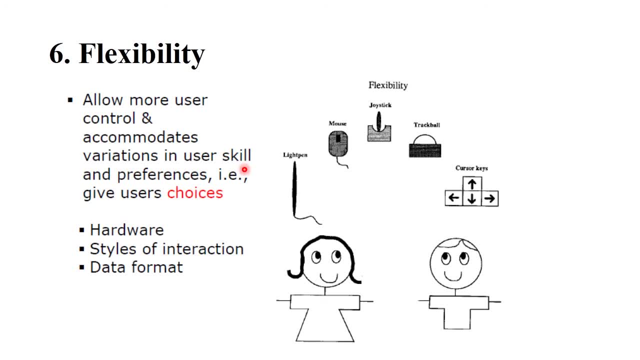 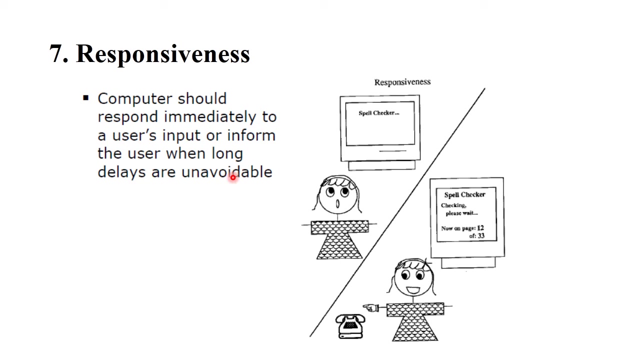 users control and accommodates it variations in user skill and preferences. that is, gives user choice. okay, the hardware styles of interaction data format for each and every persons are different, so make the product which is flexible for each and every user clear, okay. next principle of human computer interaction is responsiveness. computer 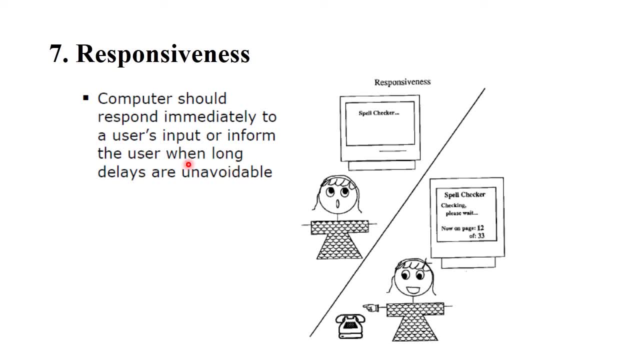 should response immediately to the users input or inform the user when long delays are unavoidable. okay, when you give particular input to the computer. computer immediately, results will be shown. computer immediately, results will be shown, right, so this is called as responsiveness: clear, okay. next principle of human computer: 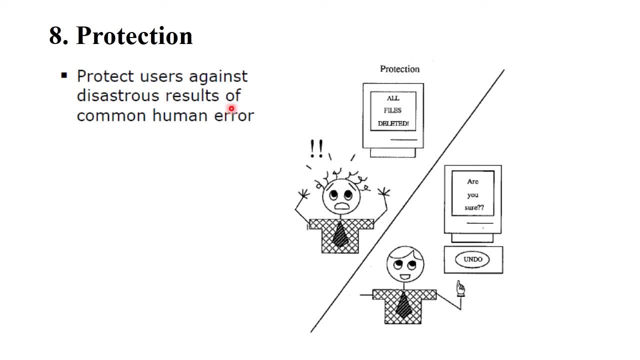 interaction is protection. protect user against disastrous result of common human error. okay, when, okay, see in this diagram, all files are deleted. okay, and see in this diagram, are you sure you have to delete this file? so this is called as protection. okay, the confirmation message shown by the system: okay, this is called as protection. okay, so this is called as protection. 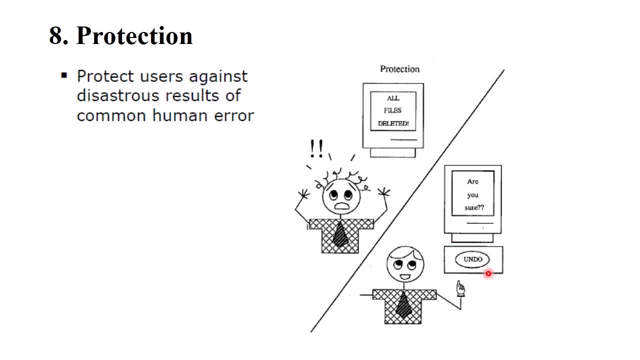 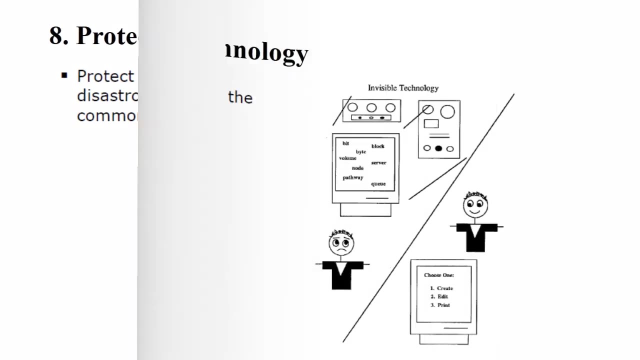 this is called as protection. clear and also undo option is also available in system. when bi-mystically you deleted, you have deleted a particular file, then by using undo option you can recover it clear. so this is called as protection, okay. next, next principle of human computer interaction is invisible technologies. no need to know technical. 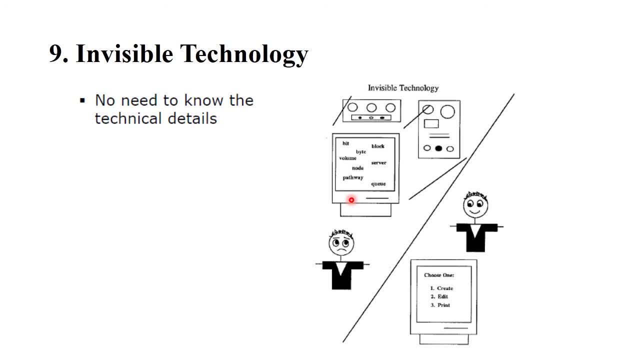 details: okay. users are very useful or usable to the front part of that particular file system. not necessary to know how particular systems are developed and how the particular functions are work. there is no need to know this in detail. information clear. so this is called as invisible technologies. okay, next. next. 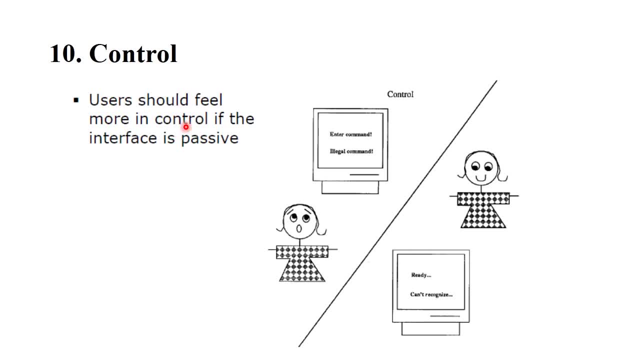 principle of human computer interaction is control. user should feel more in control if the interface is passive. okay, I already told you the interface of your product is more usable, more interactive or more attractive. okay, so you can use this interface in more ways. okay, see in this diagram this interface shows enter. 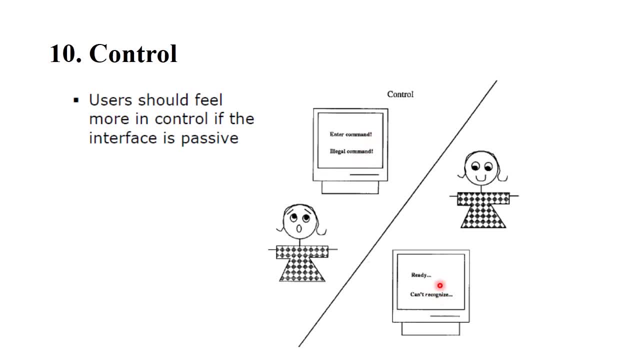 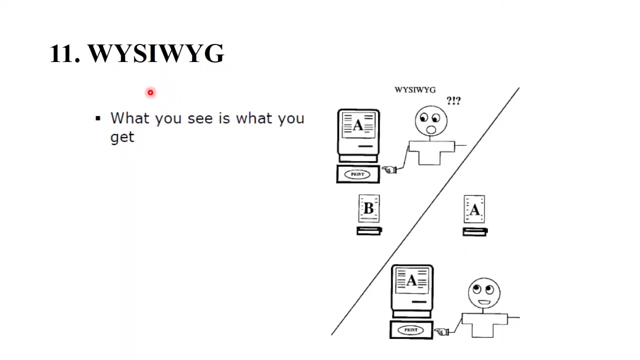 command, illegal command, and if this interface shows ready, can't recognize. okay, so this information shows in very a proper message. okay, so when you will develop your particular product, your system can be show proper information in proper words, in proper sentence. okay, so this is called as control, okay. next principle of human computer interaction. 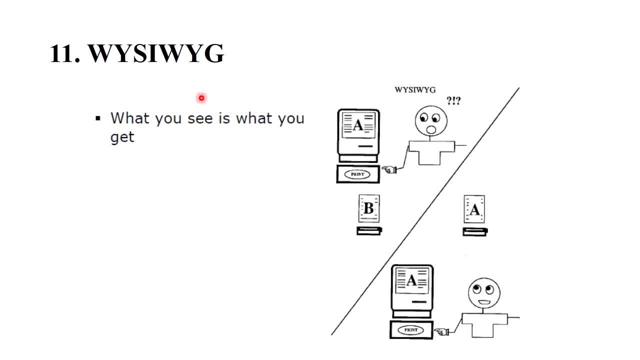 is WYSIWYG. the meaning of this word is: what you see is what you get. okay, when you print, when you, when you press the button of delete, then delete option is perform. when you say print the particular thing, then print this functionalities perform. this is called as what you see and what you get. 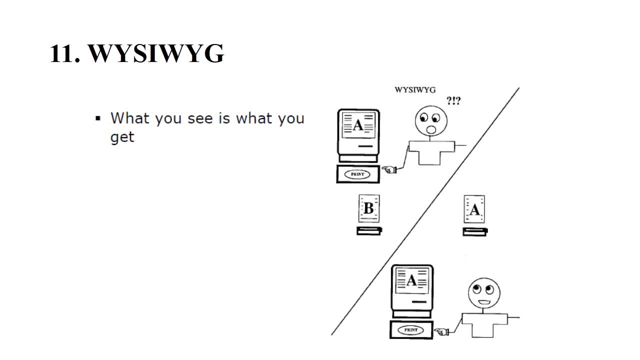 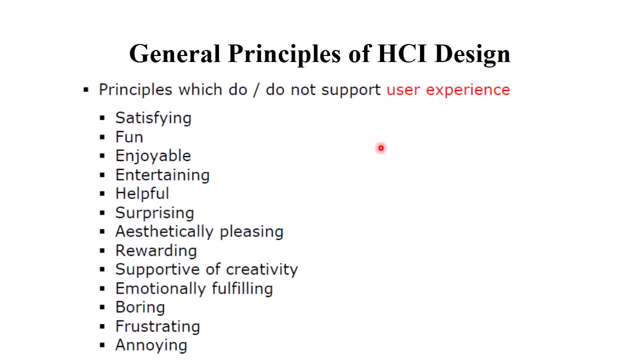 clear. this is the last principle of human computer interaction. okay, next there's some general principle of human computer interaction, principles which do or do not support user experience. okay, for example, some users may get satisfied, fun, enjoyable, entertaining, helpful, surprisingly, aesthetically pleasing, then rewarding, supportive of creativity, emotionally fulfilling, boring.